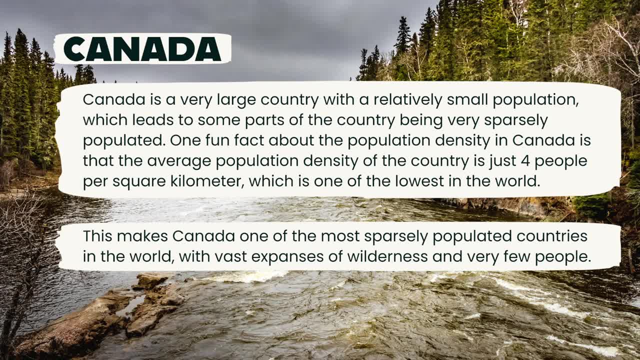 density in Canada is that the average population density of the country is just four people per square kilometer, which is one of the lowest in the world. This makes Canada one of the most sparsely populated countries in the world, with vast expanses of wilderness. 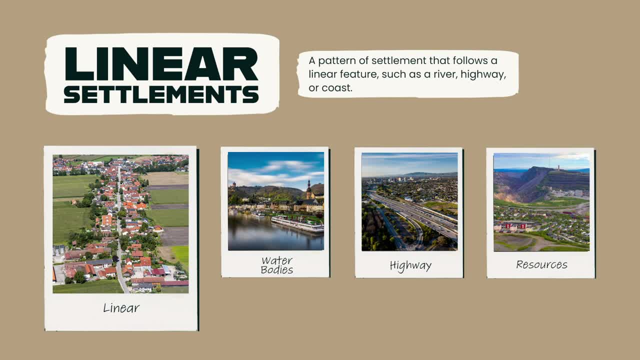 and very few people. Pattern number three is linear settlement. Linear settlement refers to a pattern of settlement that follows a linear feature, such as a river, a highway or a coastline. Linear settlement patterns can be found in a variety of contexts and can be shaped by: 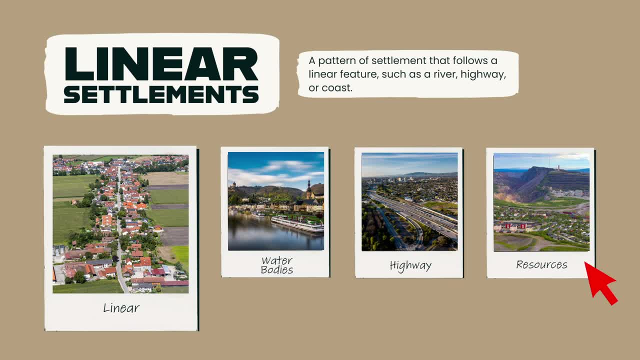 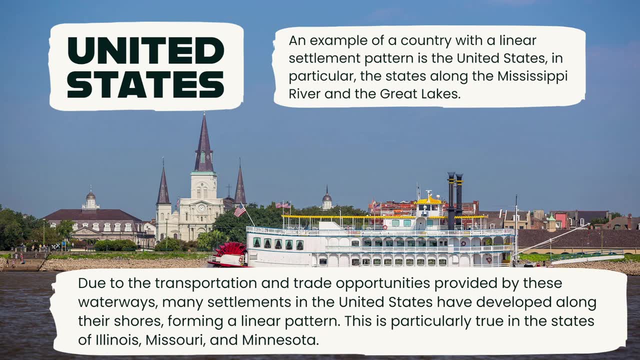 factors such as transportation networks, economic opportunities and natural resources. An example of a country with a linear settlement pattern is the United States, in particular, the states along the Mississippi River and the Great Lakes. Due to the transportation and trade opportunities provided by the United States, many settlements in the United States have developed along their shores. 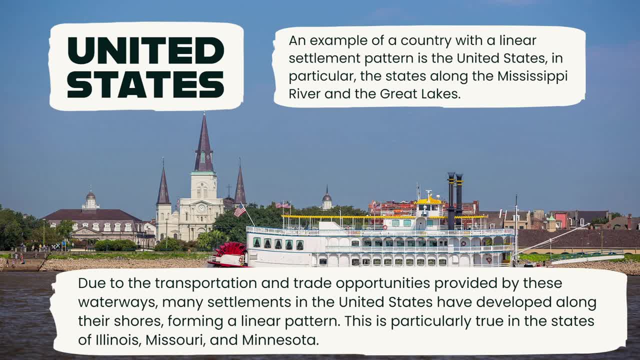 forming a linear pattern. This is particularly true in the states of Illinois, Missouri and Minnesota, where the Mississippi River and the Great Lakes have played a vital role in the economic development of the region and many towns and cities have grown up along their shores. These 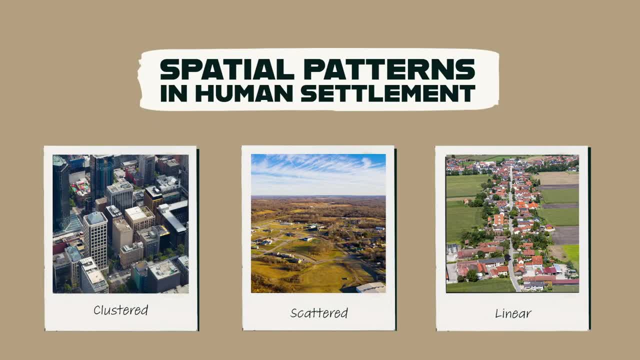 are the three main types of spatial patterns in human settlement on a global scale: Clustered, scattered and linear. Understanding these patterns can help us to understand the forces that shape the way that people live and the impacts on the environment. Now here's a 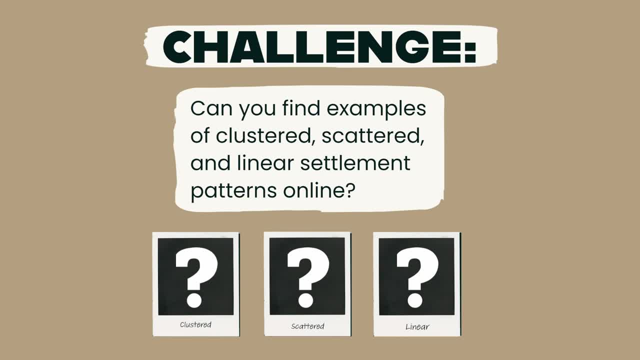 challenge for you. You'll be conducting a settlement pattern scavenger hunt. Your task is to use the internet, specifically Google Earth or Google Maps, to find examples of clustered, scattered and linear settlement patterns in different parts of the world. For each pattern: 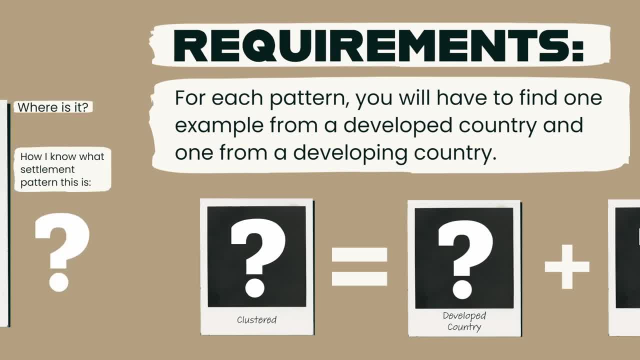 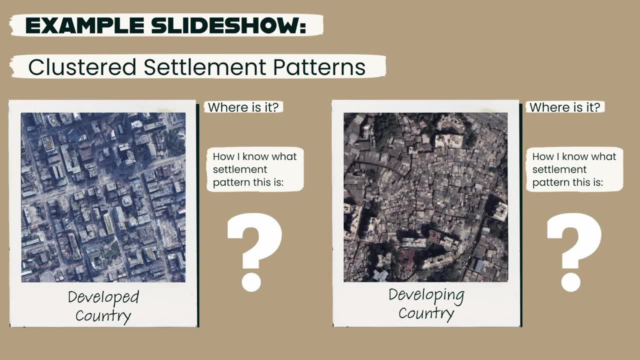 you'll have to find one example from a developed country and one from a developing country. Once you have found the examples, you'll need to take screenshots and make a short slideshow presentation. In your presentation, you'll have to explain the location of your examples. 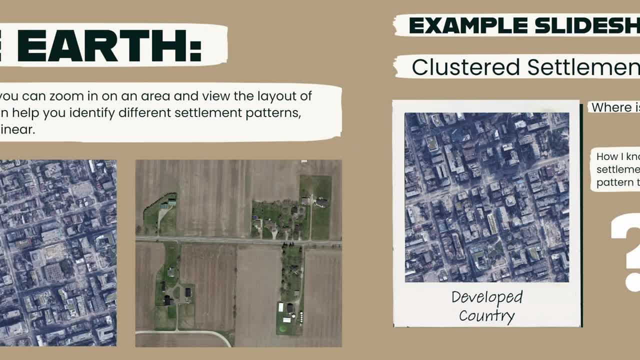 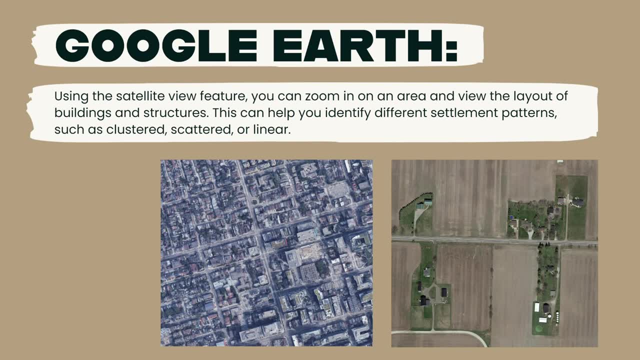 and how you know each one is either clustered, scattered or linear. Google Earth is one tool that you can use in order to find settlement patterns in different regions. Using its satellite view, you can zoom in on an area and view the layout of buildings. 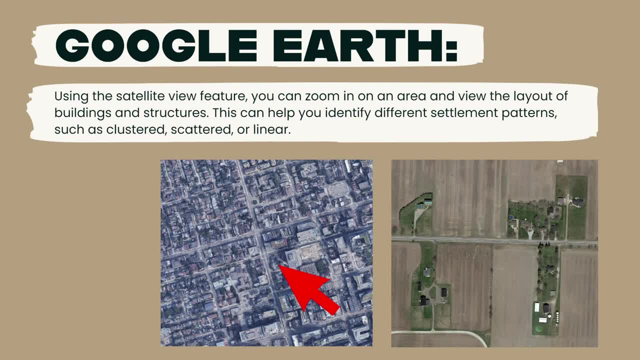 and structures. This can help you identify different settlement patterns, such as clustered, scattered and linear. For example, if you see a compact and dense arrangement of buildings and structures, it is likely that the area has a clustered settlement pattern. Good luck, 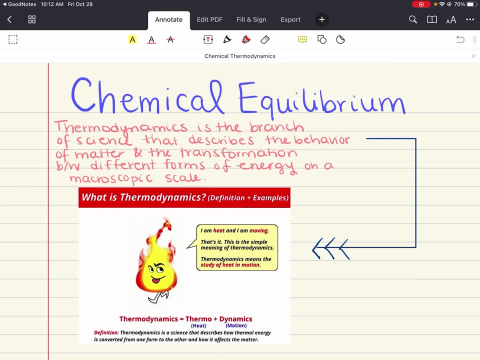 Hello everybody, my name is Iman. Welcome back to my YouTube channel. Today we're covering chapter 16 of General Chemistry, 2, and this chapter is all about chemical thermodynamics. Now, thermodynamics is the study of energy and its transformations. If you remember from Gen Chem 1,.